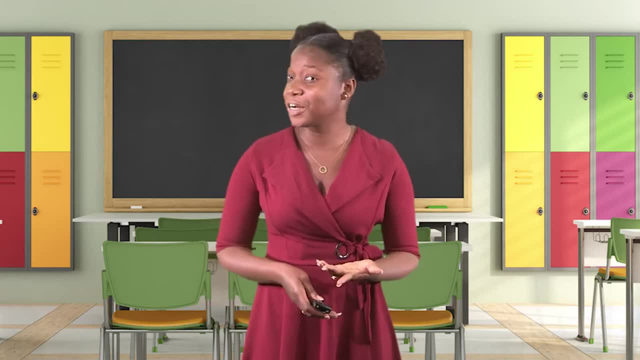 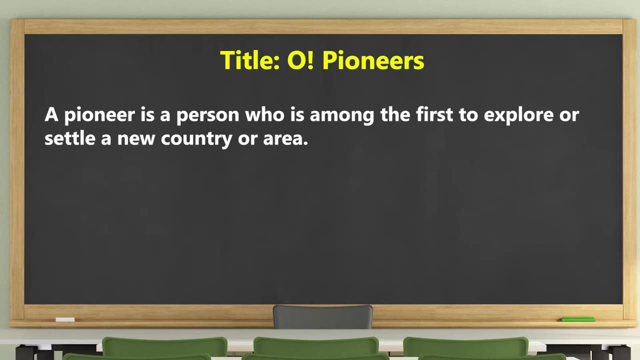 in the title. Do you know what the term pioneer means? A pioneer is a person who is among the first to explore or settle in a new country or area. I'll repeat what I'm gonna say that again: A pioneer is a person who is among the first settlers or explorers in a country. 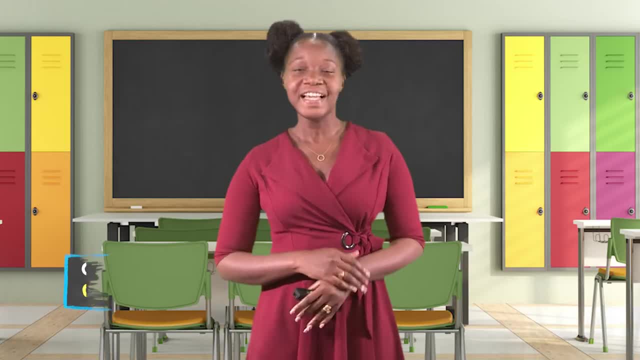 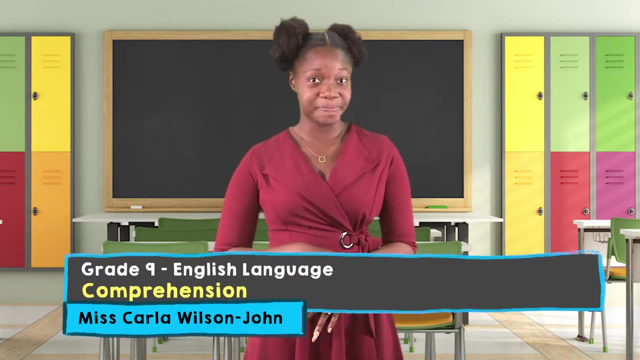 or area. Let's look at Guyana, for example. Who would you say are the pioneers of Guyana? Who would you say are the pioneers of Guyana? Who are they? All right, All right, Here we are. So what is the title say? Where are we All? Palmer-Captain- yarnu of the fosterści. or what else is there? Who is the multi topp toe Síny-fiviáisェ, Who is the famous good child of life? Where is the star of this holiday that you love, The star of the activity that you are? you love, Good, Good. Well then, first, what we're gonna say is the pioneer of Is Houla, There's a certain 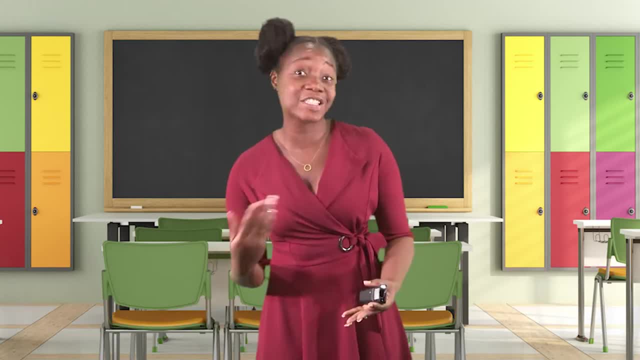 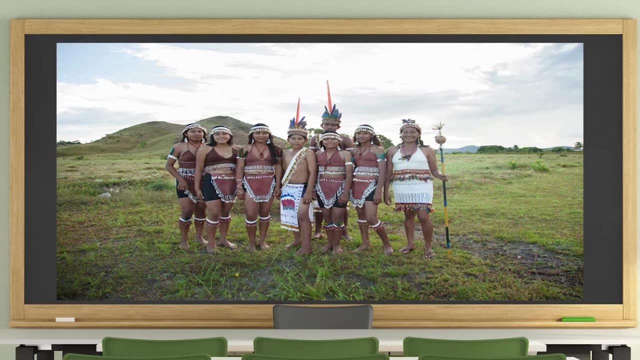 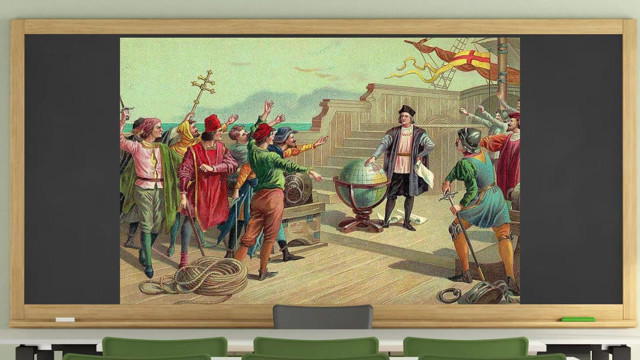 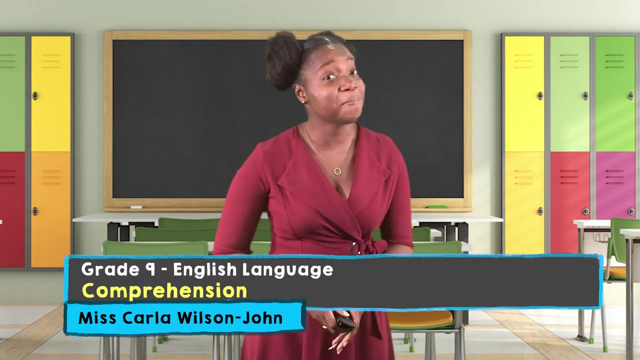 say, are the first settlers or explorers. Now, we know the Amerindians were the first persons to come and settle on our land And then the Europeans came as explorers. Do you know the pioneers of any other country? Do you know the pioneers of any island? Maybe Trinidad and Tobago, or Barbados? 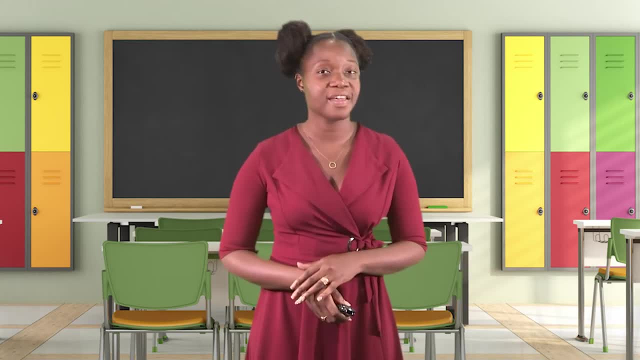 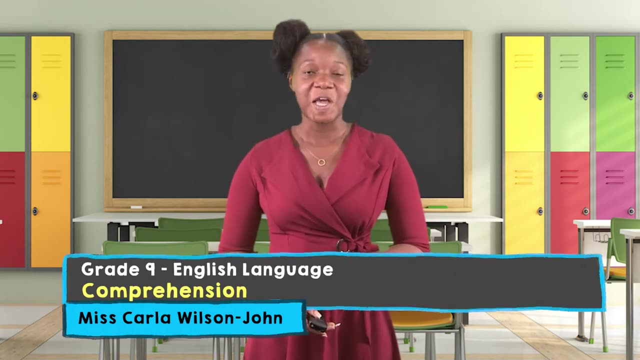 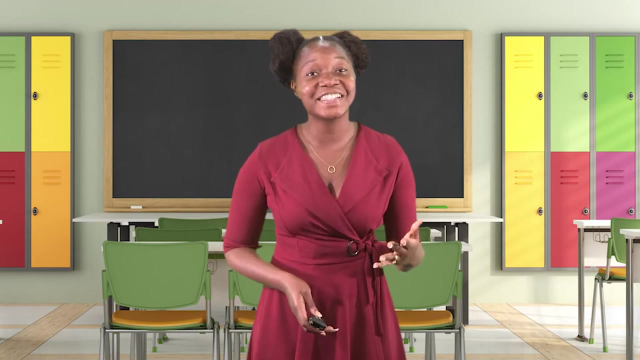 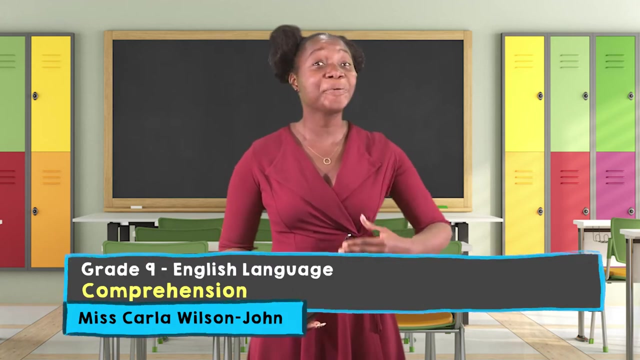 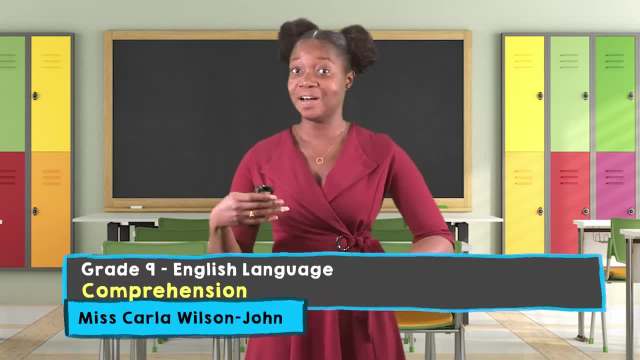 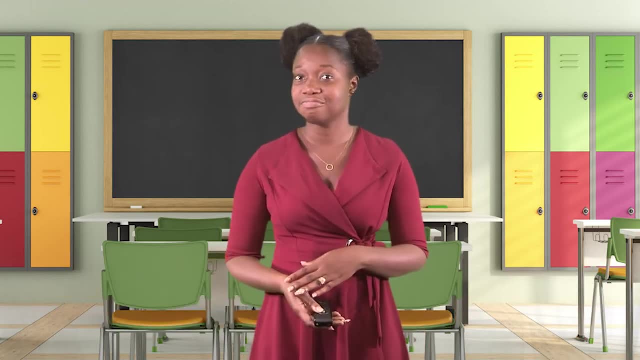 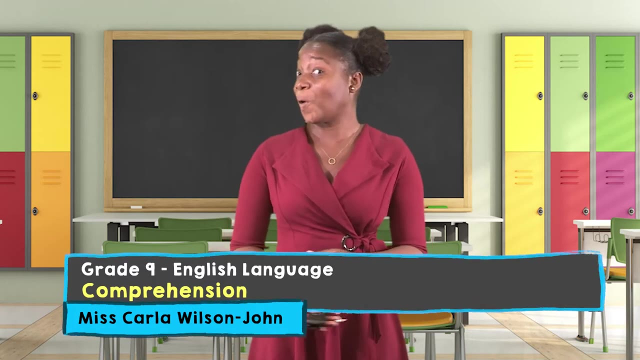 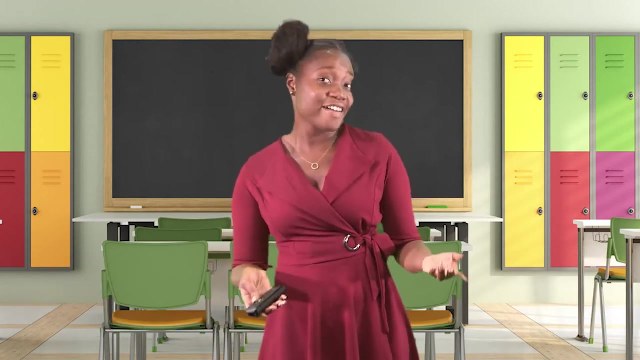 What are they going to establish there, as they go on this new island or this new country? What will they eat? What do you think we will find as we read this passage? Oh, pioneers, could you predict the name of the characters? All right, so that was prediction. 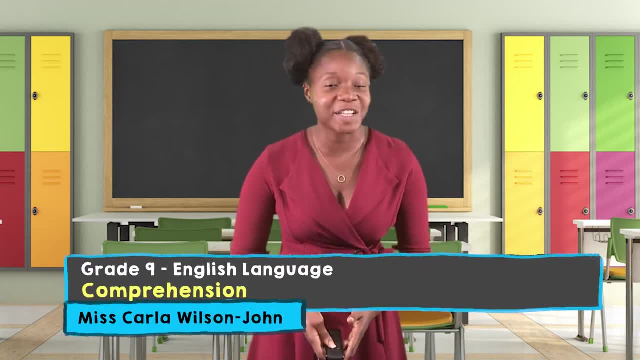 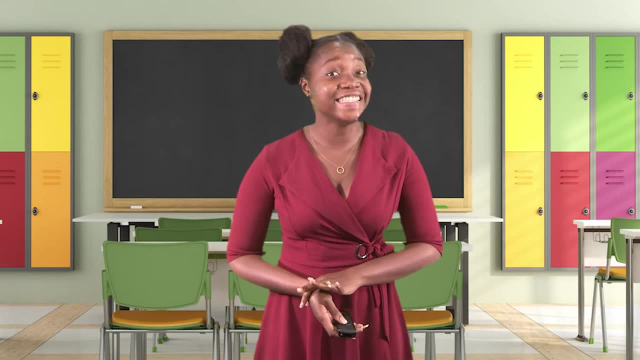 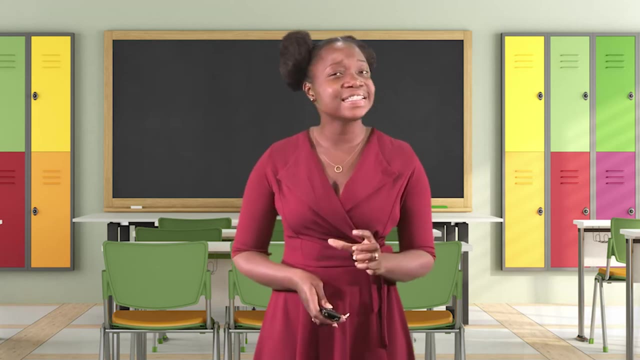 Now let's get into the actual story. Oh Pioneers was written by Willa Cotter in the year 1910.. It is a novel, so it is really long, But in this lesson we're only going to read a short passage from it. 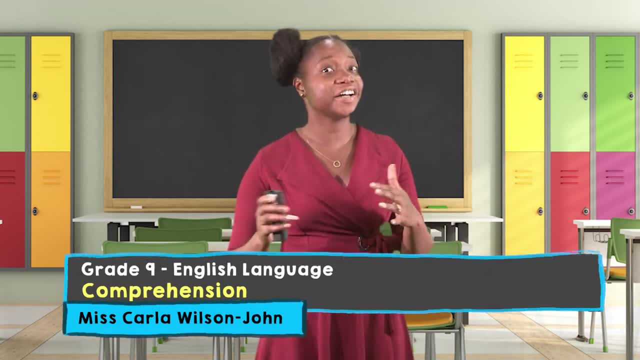 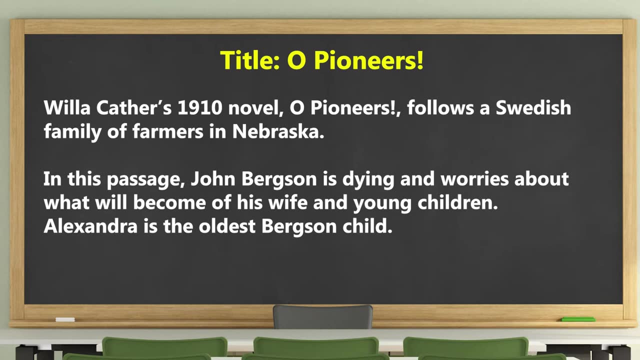 So you may not get the full gist of the entire novel. So I want to give you a little background just before we read In this passage. John Bergson is dying and worries about what will become of his wife and his children. Alexandra is the oldest Bergson child. 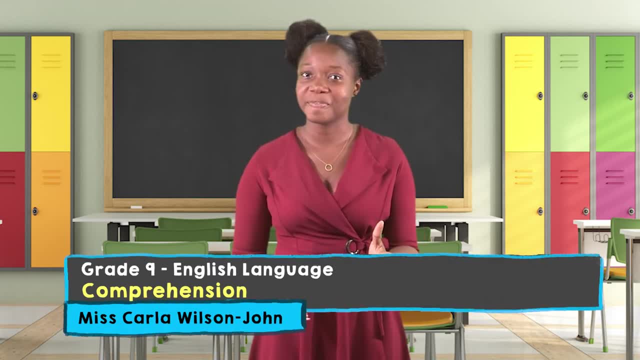 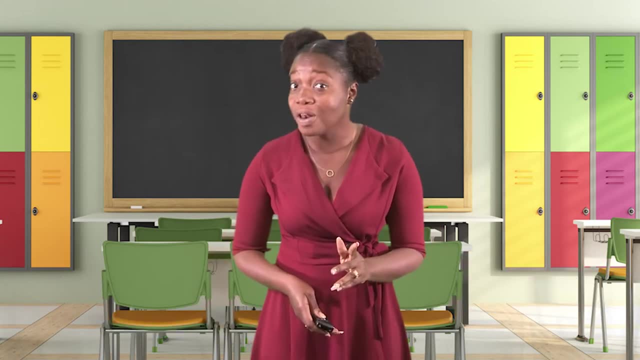 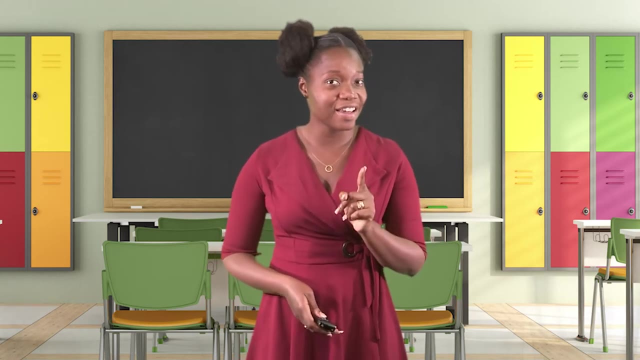 So let's see what this passage is all about. Remember, we are reading it for comprehension, So you have to follow along and you have to try your best to understand. understand, because after we read, we're going to discuss And I have a question or two to ask you. 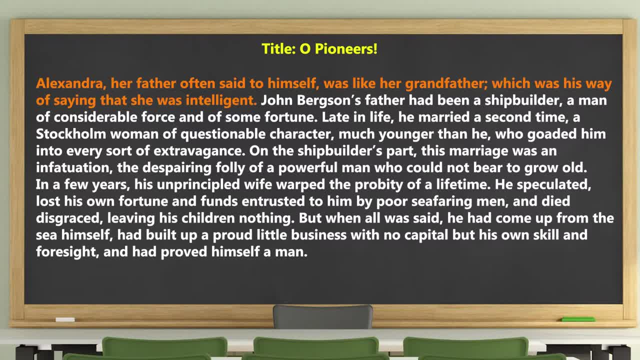 Let's begin. Alexandra, her father often said to himself, was like her grandfather, Which was his way of saying that she was intelligent. John Berkson's father Had been a shipbuilder, a man of considerable force and of some fortune. Late in life he married. 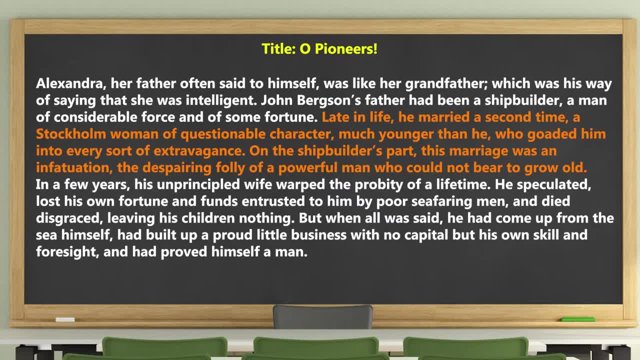 a second time, a Stockholm woman of questionable character, much younger than he, who goaded him into every sort of extravagance. On the shipbuilder's part, this marriage was an infatuation, the despairing folly of a powerful man who could not bear to grow old In a few. 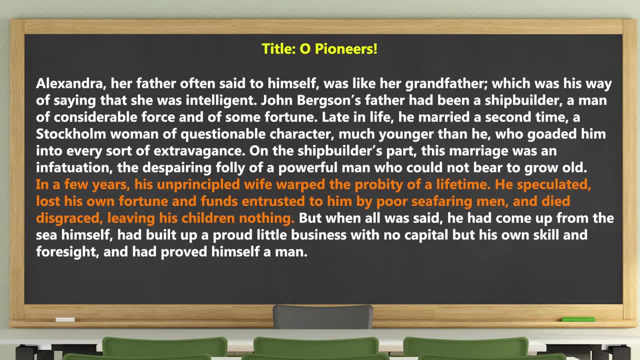 years his unprincipled wife warped the property of a lifetime. He speculated, lost his own fortune and funds entrusted to him by poor seafaring men and died disgraced, leaving his children. But when all was said and done, he had come up from the sea himself, had built up a proud 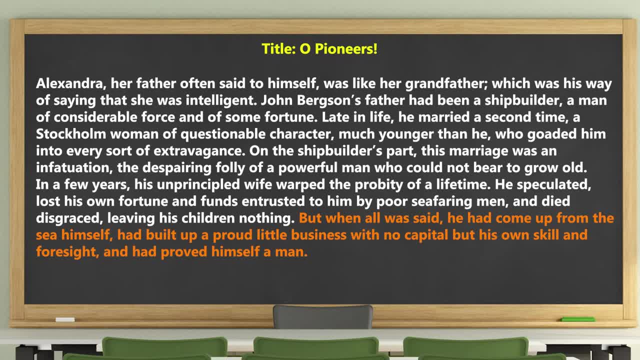 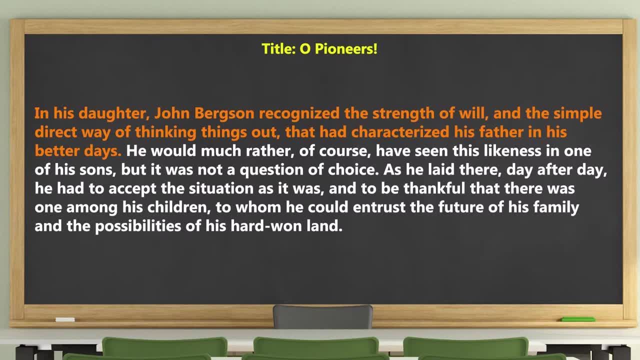 little business with no capital but his own skill and foresight, and had proved himself a man. In his daughter, John Bergson, recognized the strength of will and the simple, direct way of thinking things out. John had said that his father had become a man of wisdom by the fact he had not hired. 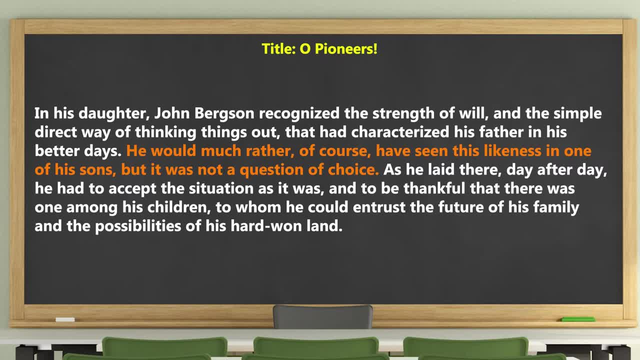 a woman to bring in wealth and wealth of the rich. He had seen his life as a child of a rich man who was looking after his very own family. He had seen that he could afford to buy and stay in the US and live in this beautiful 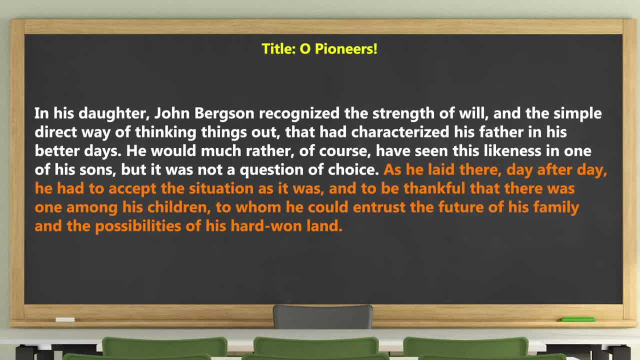 country. As he lived there, he knew that there was someone who could be a better man. It was a man of wisdom. This was a man of wisdom of his family and the possibilities of his hard-won land. All right, students. so this was the passage. 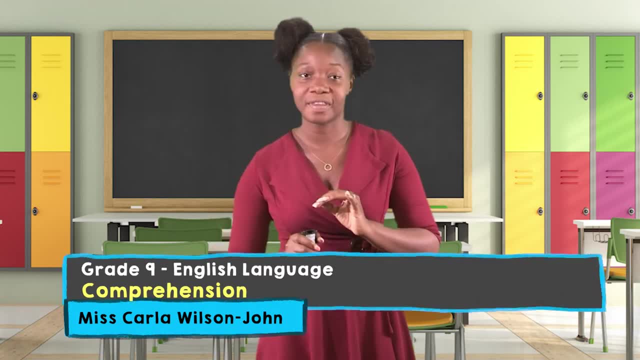 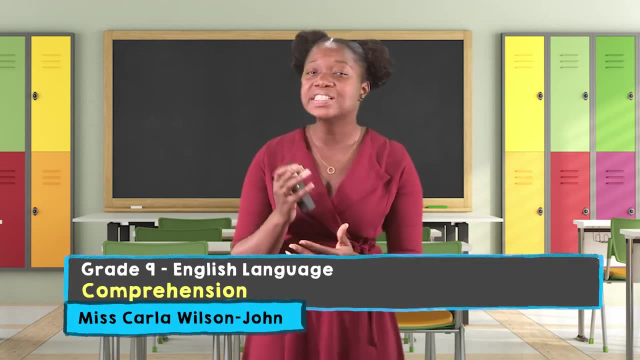 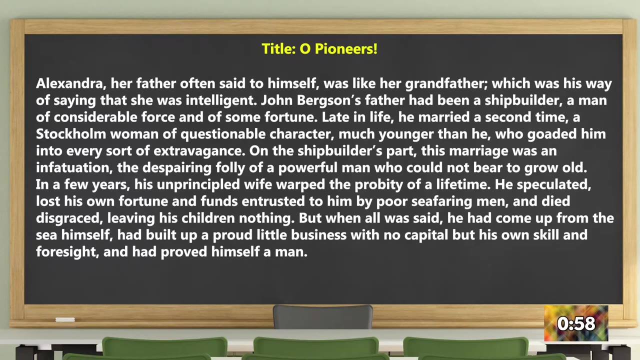 Take a minute, peruse it for yourself. We're looking for names of persons, who the narrator might be. what are we talking about? What is happening in this passage? All right, we're looking for names of that person, and who would that be? 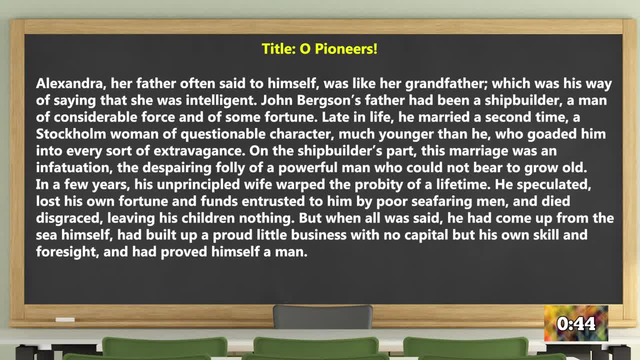 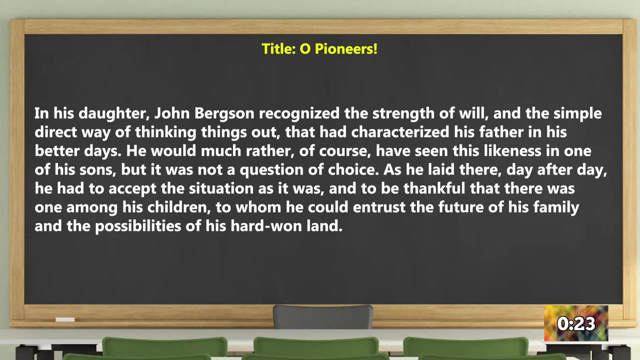 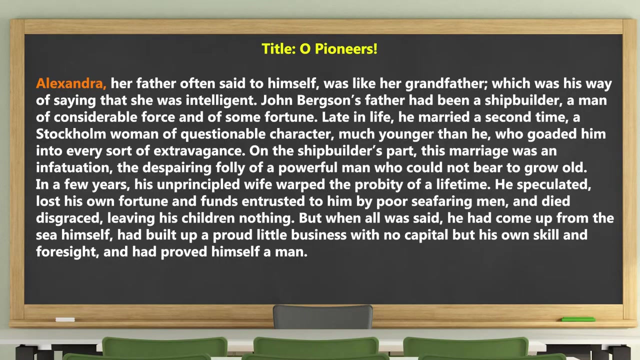 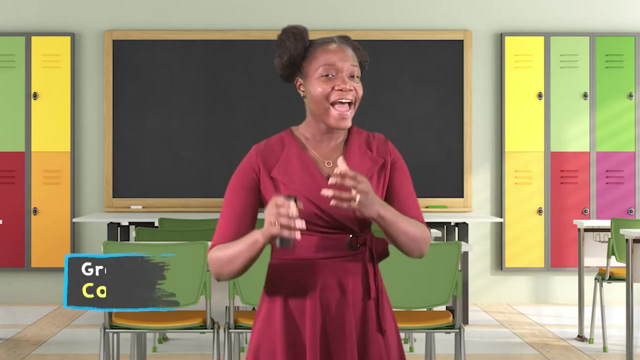 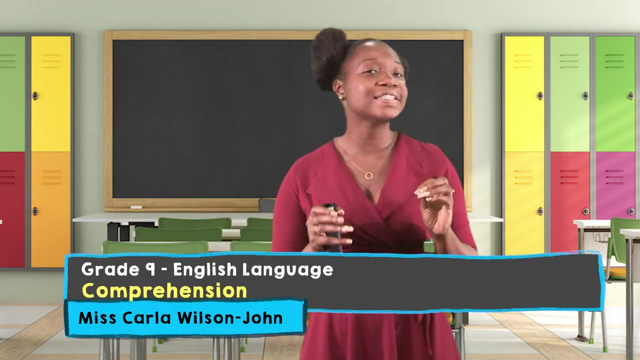 And what kind of person might it be? Let's have the narrator say it for us: Here we go, Here we go, here we go, Hey, hey, hey, hey, hey, hey, hey. Thank you, Thank you. 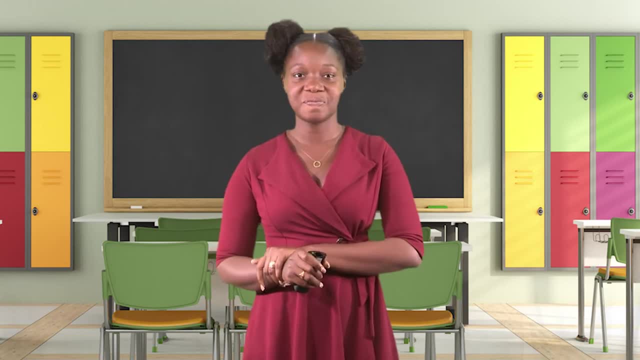 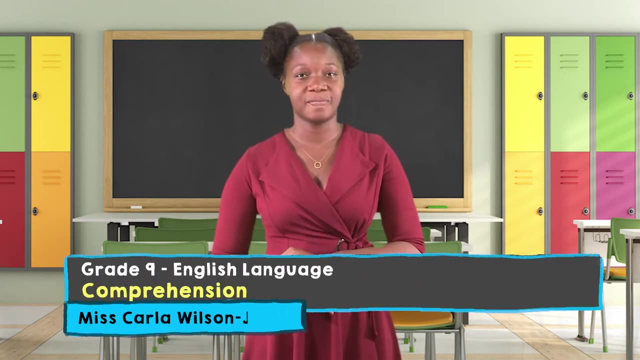 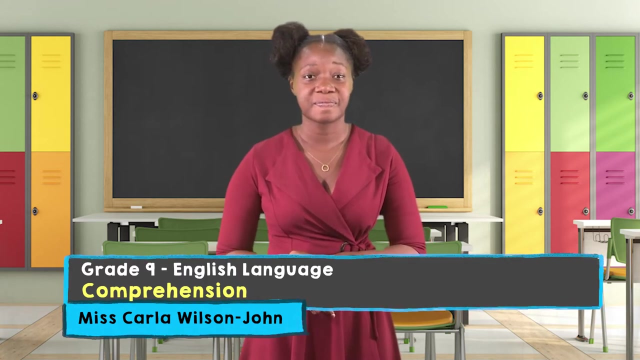 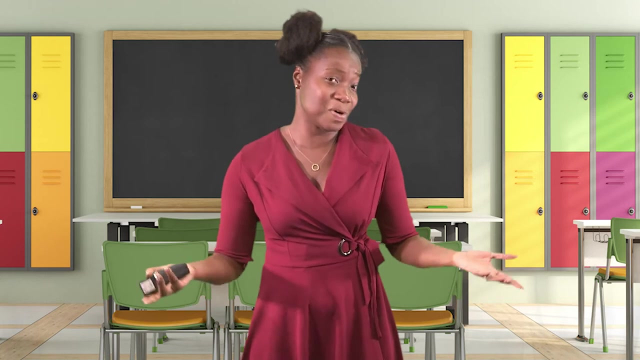 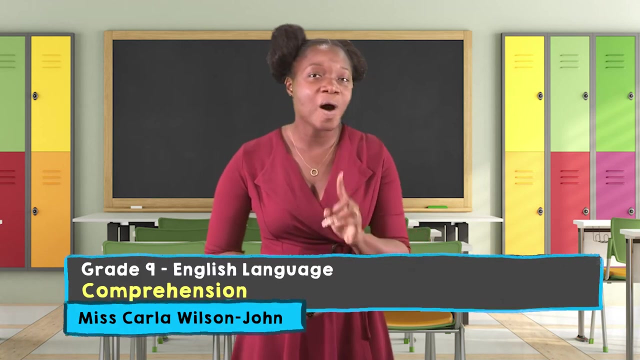 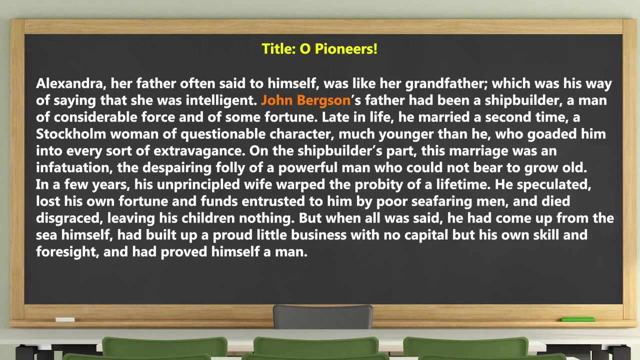 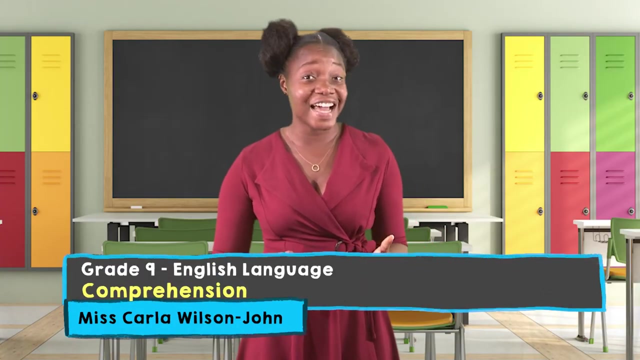 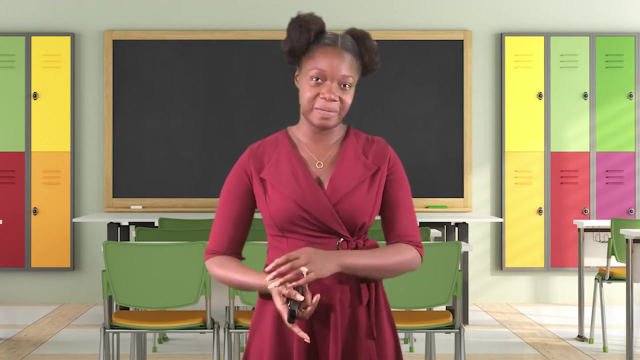 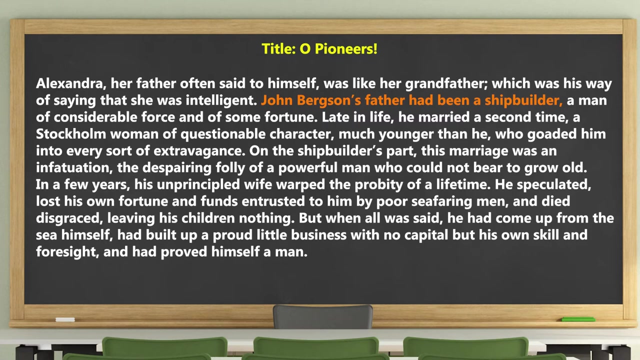 Thank you. And what is her father's name? John Berkson. Yes, My next question to you will be: what was Alexandra's grandfather's occupation? What did he do for a living? He was a ship builder. Good job Now a long life. we see he had various experiences. 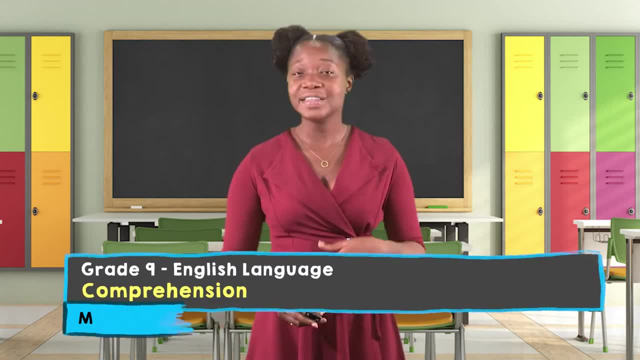 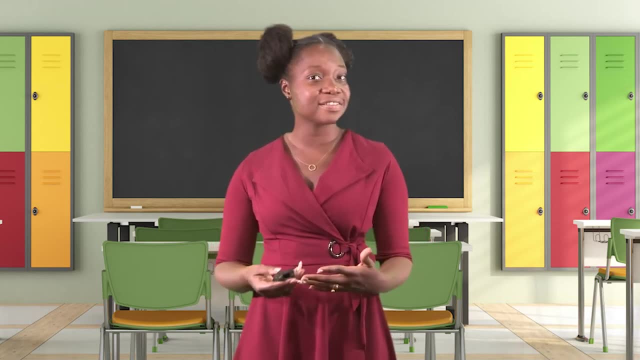 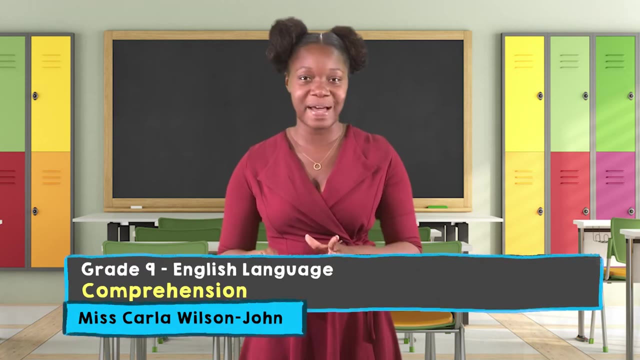 We see that he married twice And the wife that he had, his second wife, was younger than he was And she caused him to do some things. Yes, But my most important question to you, based on this passage, is: did he get married to his second wife? 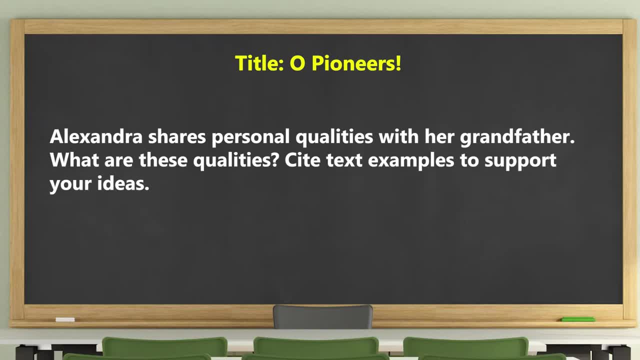 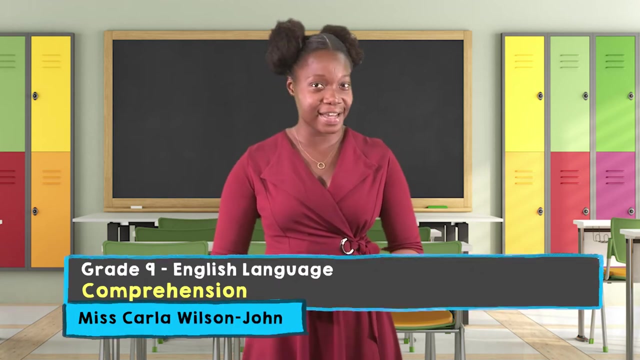 Yes, Alexandra shares personal qualities with her grandfather. What are these qualities? Cite text examples to support your ideas. I go to question again: Alexandra shares personal qualities with her grandfather. what are these qualities? cite text examples to support your ideas. so here you would have to refer to the text, always refer to the text if you are not sure. 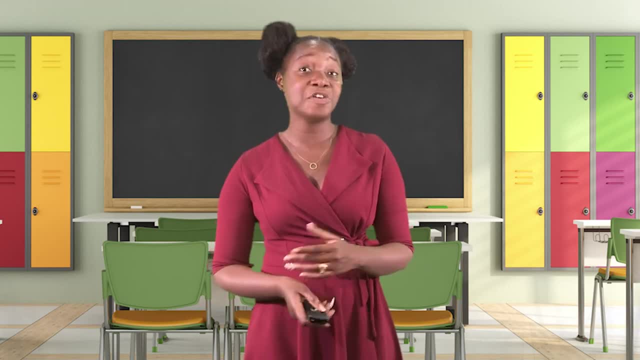 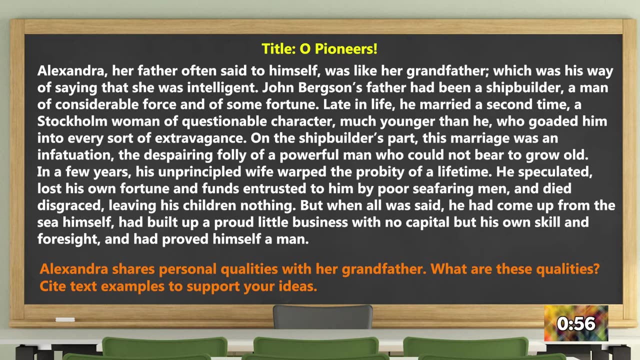 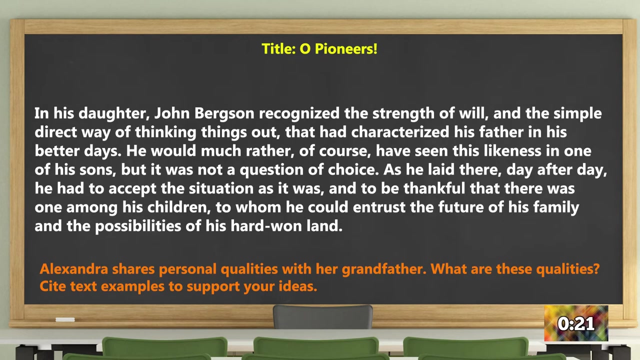 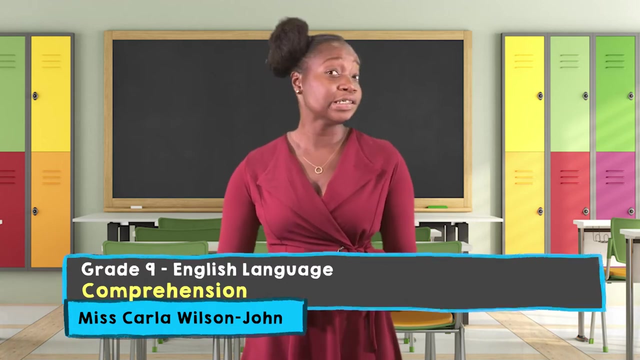 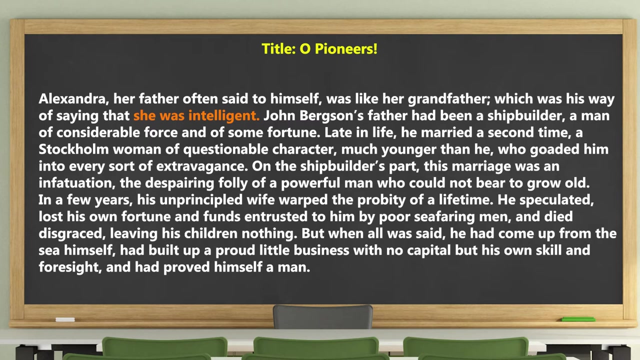 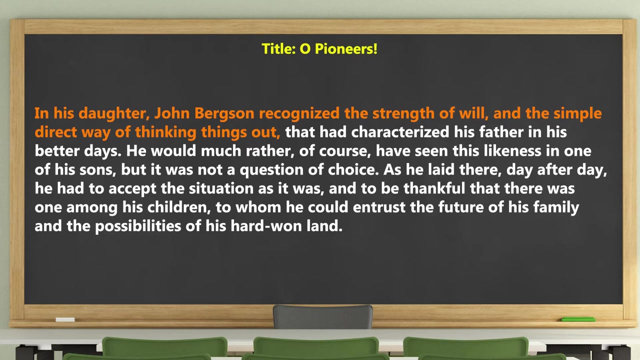 always refer to the text if you cannot remember the answer, you good. so where and how did the father compare alexandro to his father? and the answer would be: alexandra was intelligent, she possessed a strong will, it was as though she had fortitude, won't you say? and she had a simple direct way. 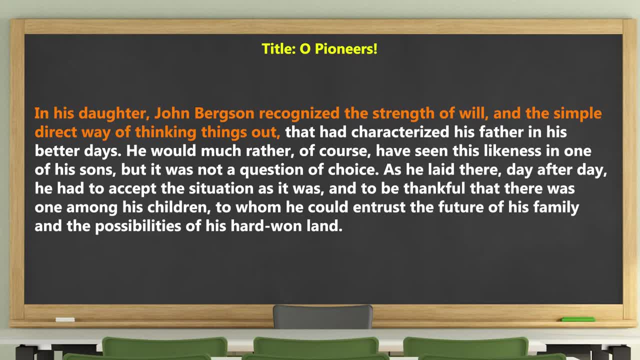 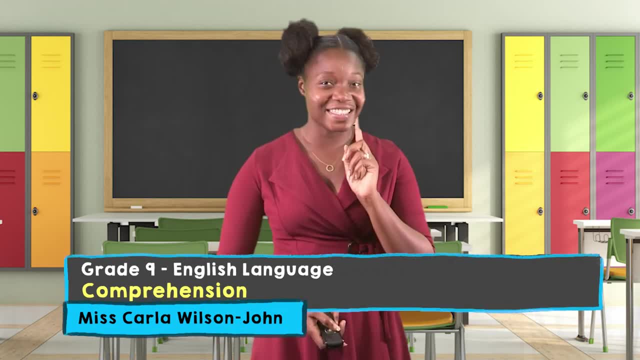 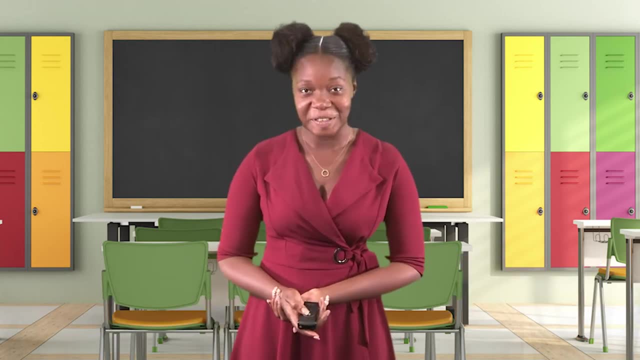 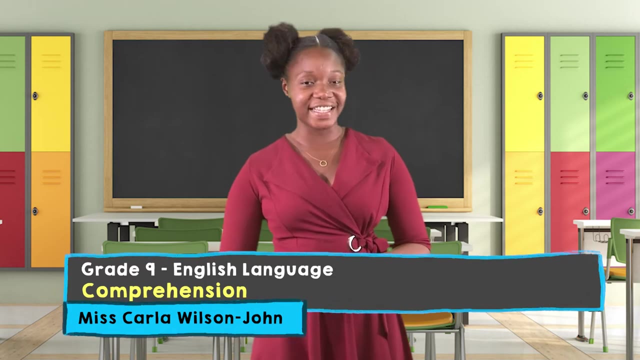 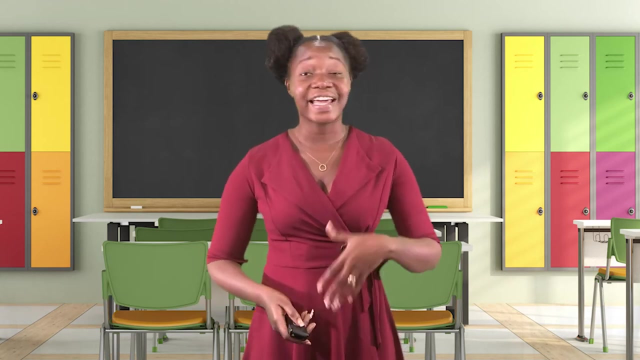 of thinking things out. she was a good thinker. so if the father were to die anytime soon, he knew for sure that alexandra would be there to help the family through any challenge. good, and now for our second story. this passage is titled the tell-tale heart. and remember, like I said, 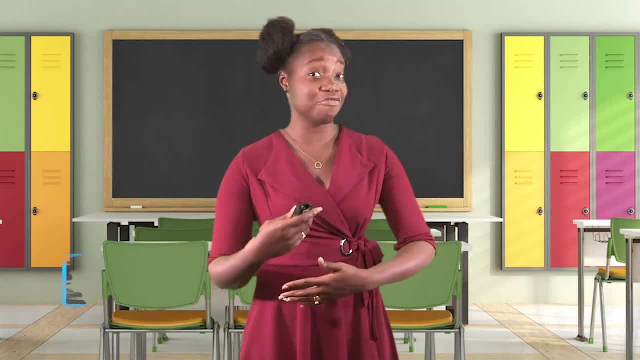 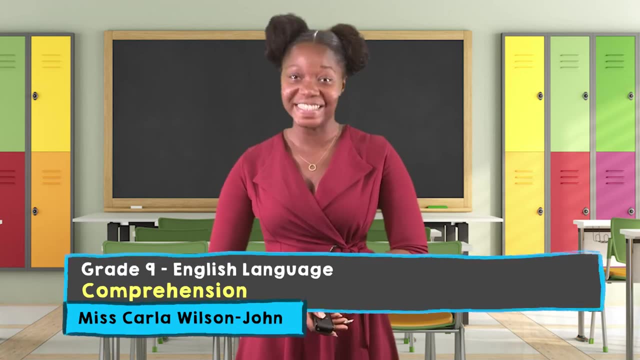 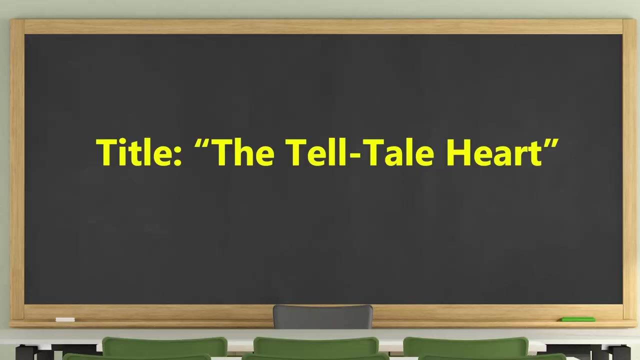 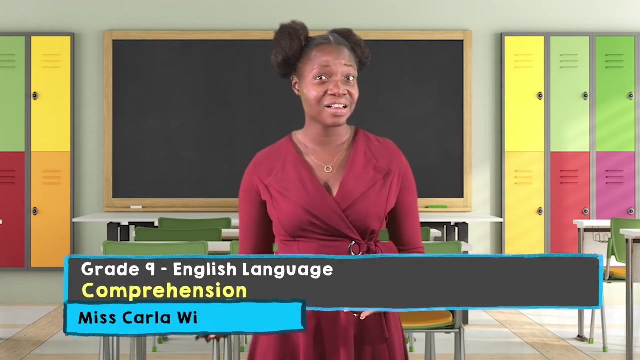 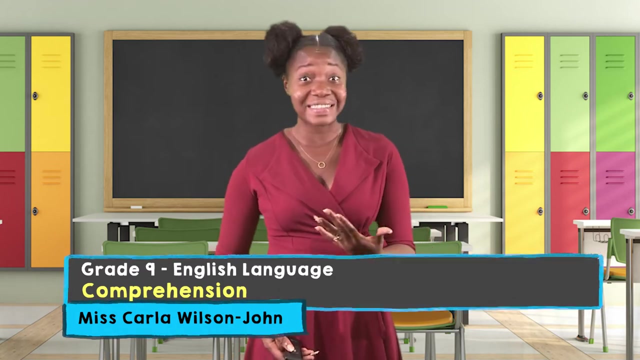 before, just before we begin to actually read the story, we must look at the title and make predictions. yes, so when we talk about the tell-tale heart, exactly what are we talking about? it's a heart telling a story, a tale? is it saying something? is the heart whispering and it wants us to feel what it's saying we? 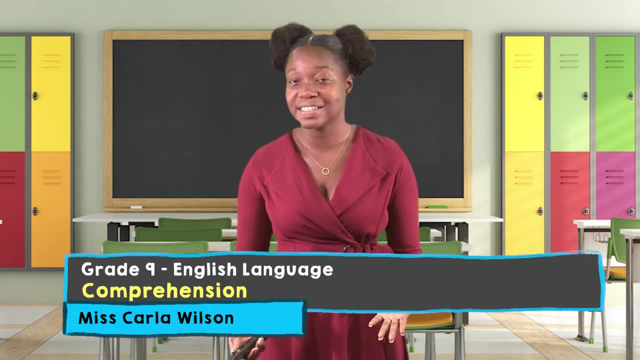 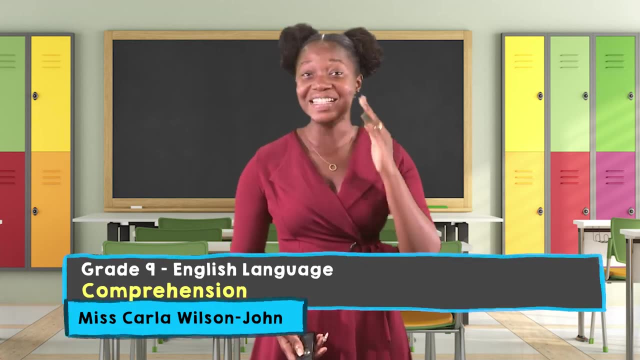 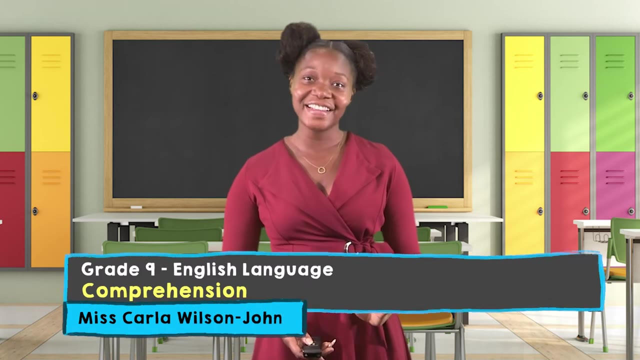 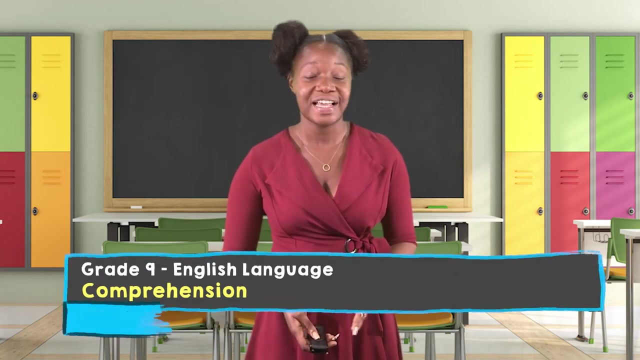 don't know, but that's what prediction is all about. you may never be sure, because you would not have read this story before, but we can only think and imagine what is going to happen. so the tell-tale heart is written by Edgar Allen Poe. this is one of his famous short stories and again, we're only going. 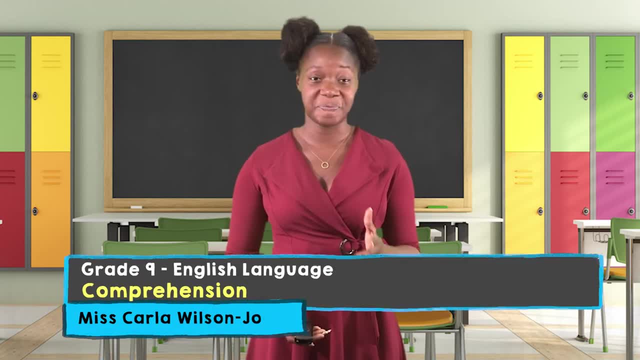 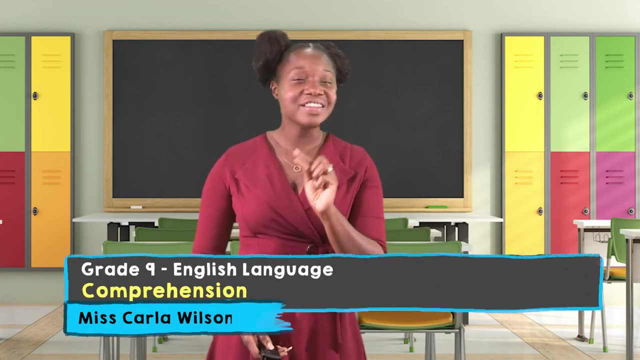 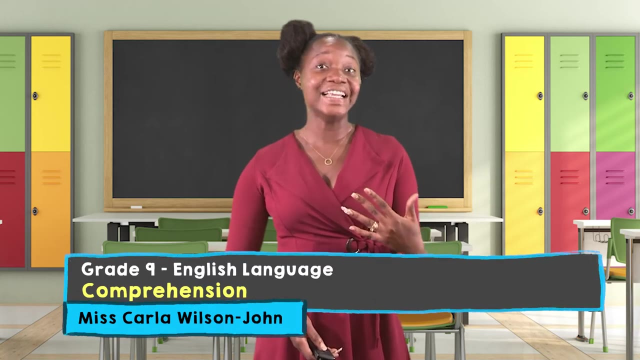 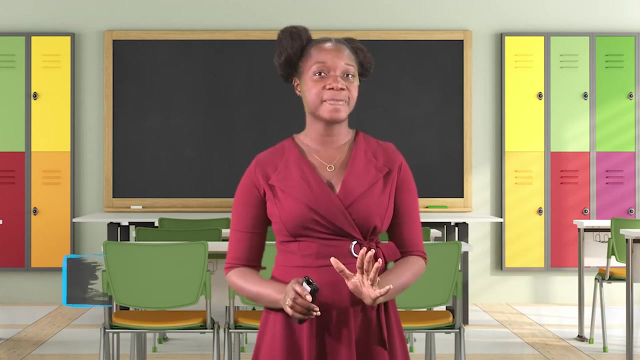 to read a few paragraphs from the story. right, just opening paragraphs we're going to read. let's go As we read this story. I would like you to listen and follow. Listen for my enunciations and pronunciations. I would like you to gather, as we go through this one, that you don't just 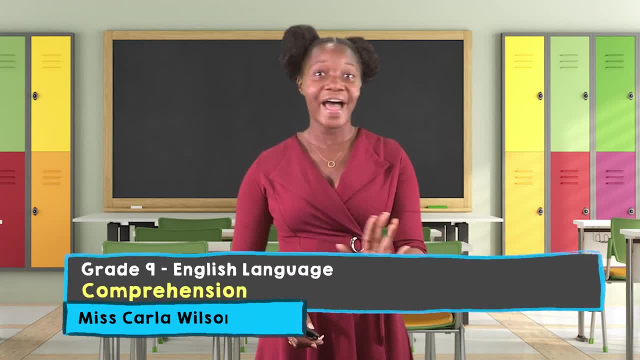 read what you see by calling words, identifying words and your phonics is good. As you read, you ought to raise your voice and lower your voice. You need to change your pitch. Make reading fun. You ought to observe punctuation marks and enjoy the language as you go through. 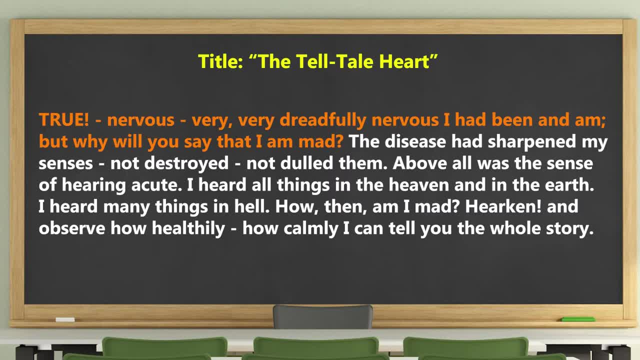 So let's have fun with this one. True Nervous, Very, very dreadfully nervous, I had been and am. But why will you say that I am mad? The day this disease had sharpened my senses- Not destroy them, Not dull them- Above all was 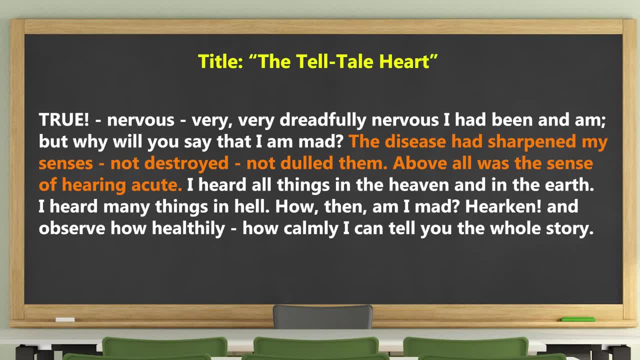 the sense of hearing acute. I heard all things in the heaven and in the earth. I heard many things in hell. How then am I mad, Hearken, and observe how healthily and calmly I Vadha produk, dealt with? sorrow and light had cadaverally trap valeur in him. What was the hurt for? for God. The curse upon me. Not wicked schon was mustn't superb. Look for love. to tear madam's will at him. If he were evil, he would be a self free. that lay him bare again. Cain had fainter with you. I will add veneration. From who am I mad? The curse upon you, See. 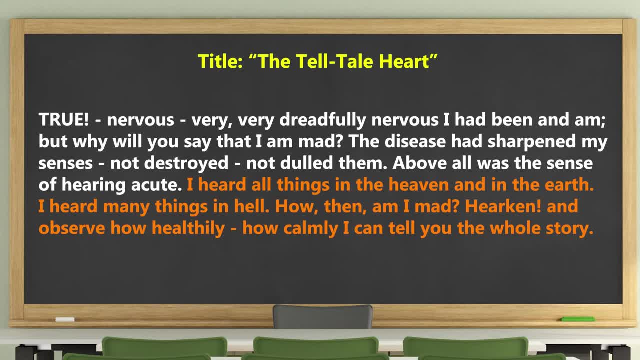 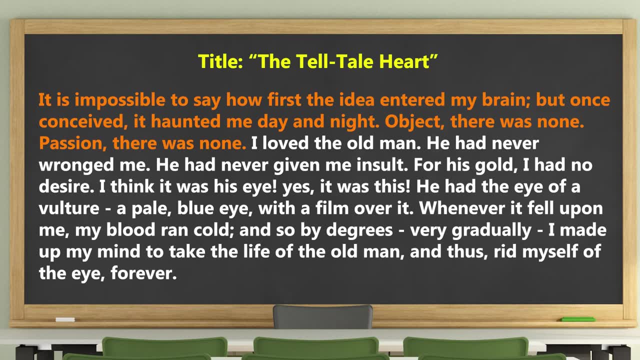 can tell you the whole story. It is impossible to say how. first the idea entered my mind, but once conceived, it haunted me day and night. Object: there was none. Passion, there was none. I loved the old man. He had never wronged me. 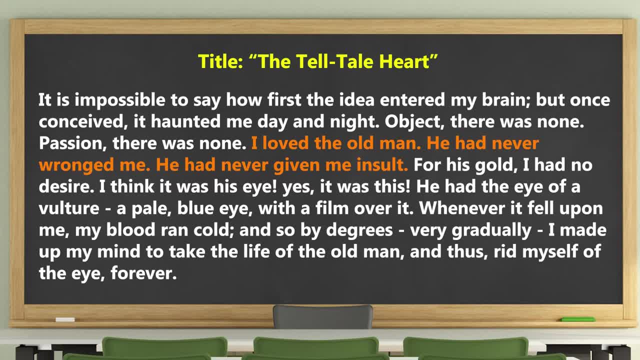 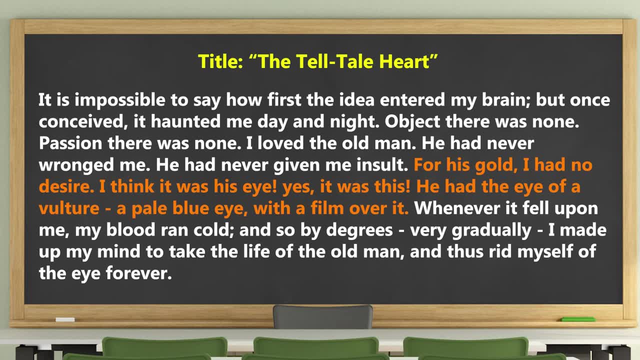 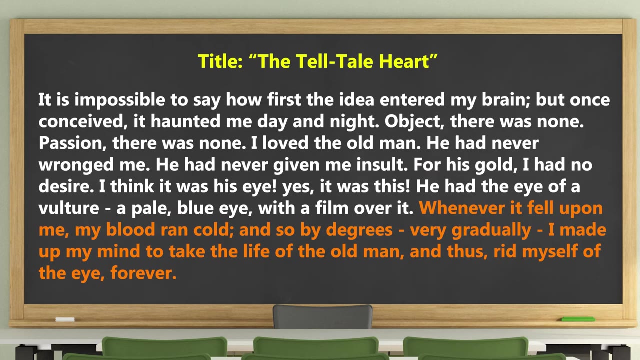 He had never given me insult For his gold. I had no desire. I think it was his eye. Yes, it was this. He had the eye of a vulture, A pale blue eye with a film over it. Whenever it fell upon me, my blood ran cold. 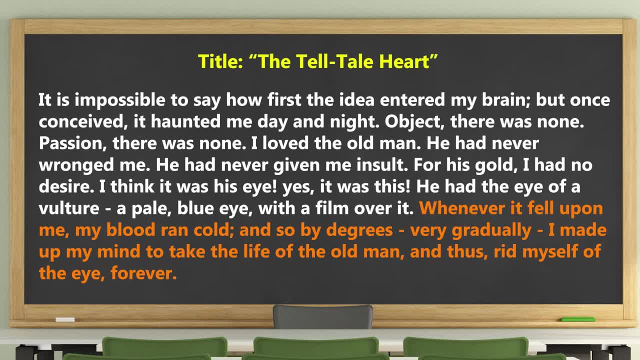 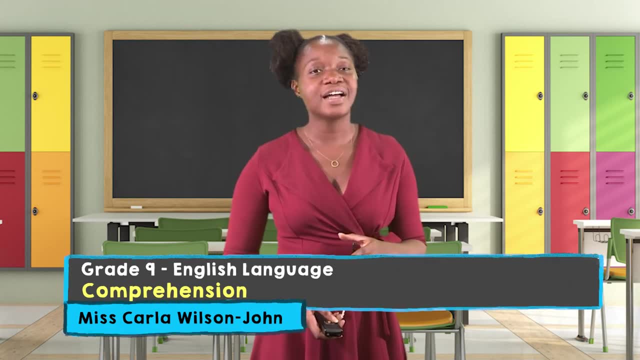 And so, by degrees, very gradually, I made up my mind to take the life of the old man and thus rid myself of the eye forever. All right, So this was a sharper piece of passage, Not as normal as we would like to think it to be. 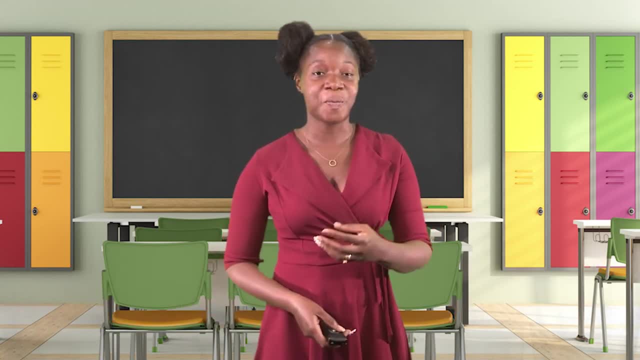 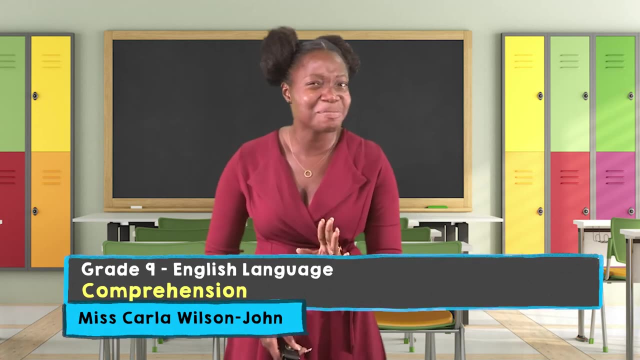 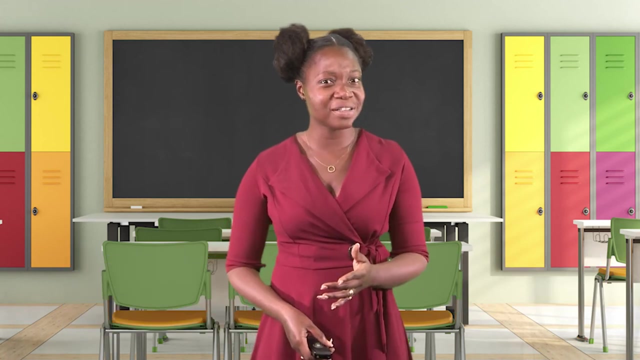 But here we're actually met with a person who is being accused and questioned of his sanity And he's trying to say that no, he's not mad, He is quite normal in his thinking. Do you think he's normal? How I read it based on the punctuation marks: 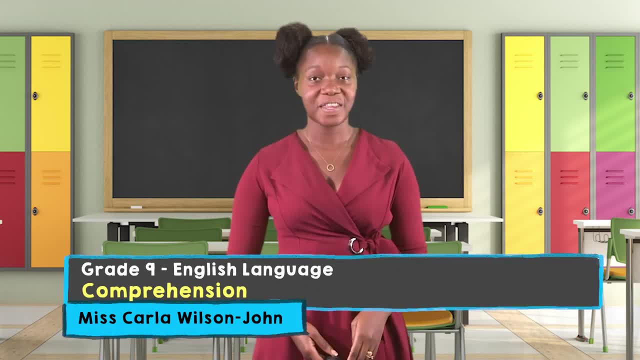 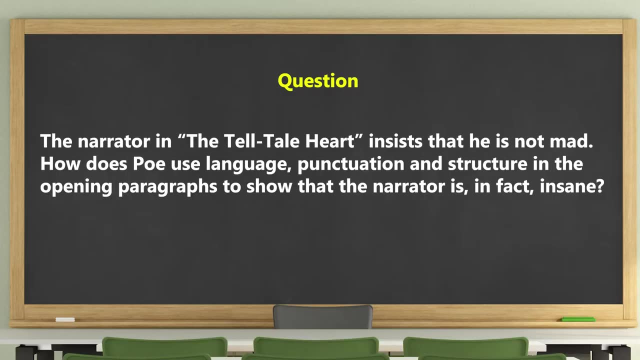 is this the way a normal person speaks? So I have a question for you based on this passage. The narrator in the tell-tale heart insists. The narrator in the tell-tale heart insists. The narrator in the tell-tale heart insists. 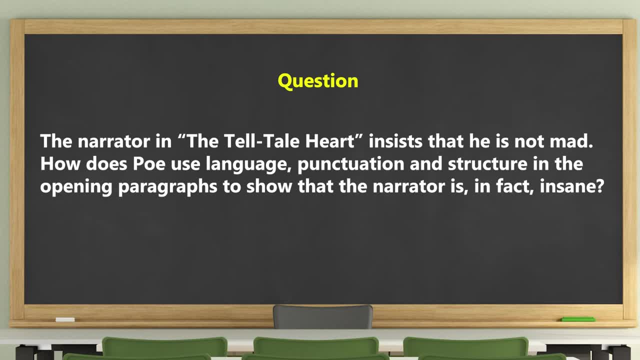 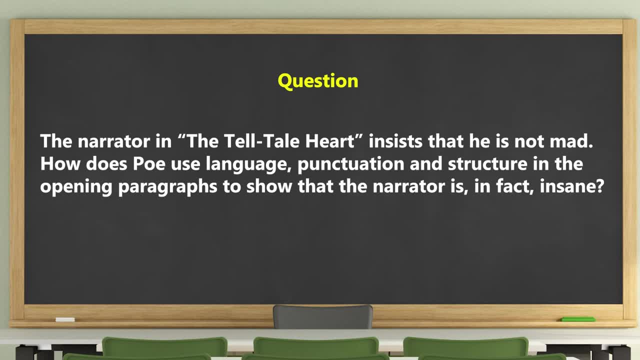 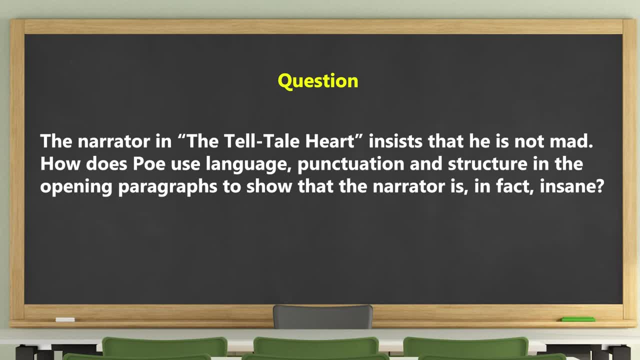 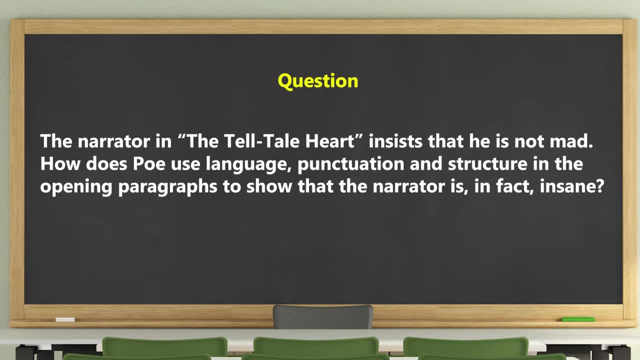 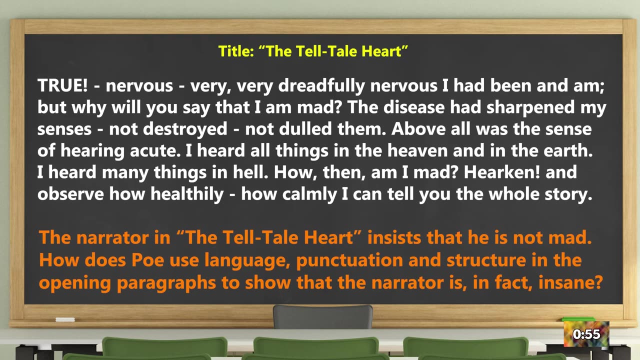 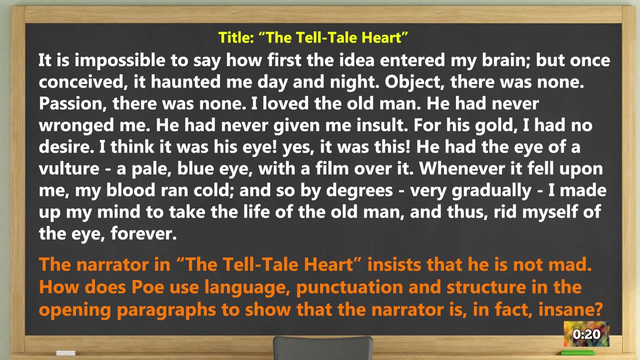 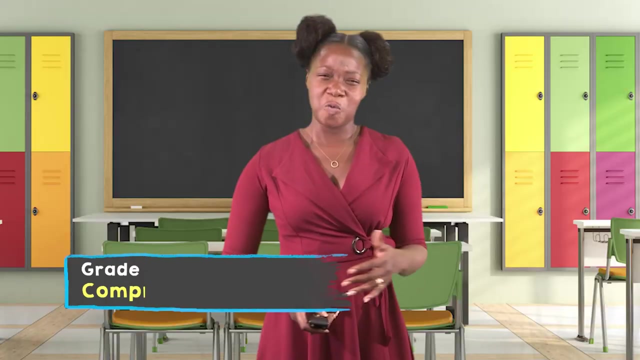 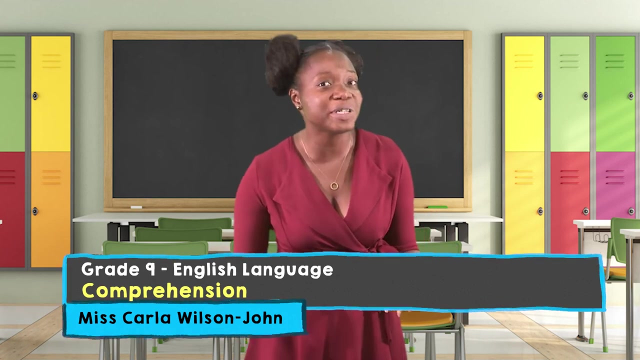 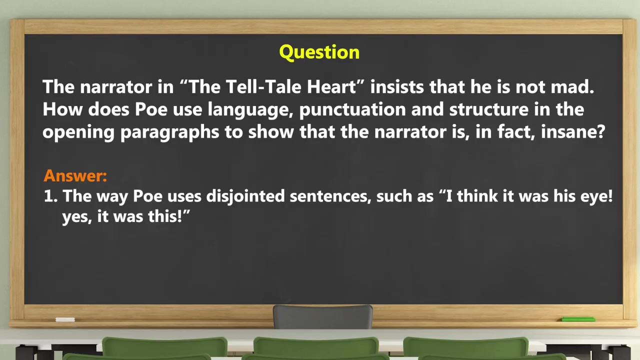 in the paragraphs to show that the narrator is in fact insane or mad. Remember to always go back to the passage. © BF-WATCH TV 2021. © BF-WATCH TV 2021. Yes, so the very way the lines are set up, disjointed sentences such as I think it. 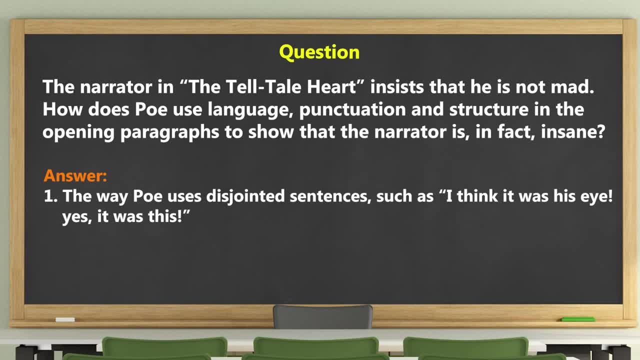 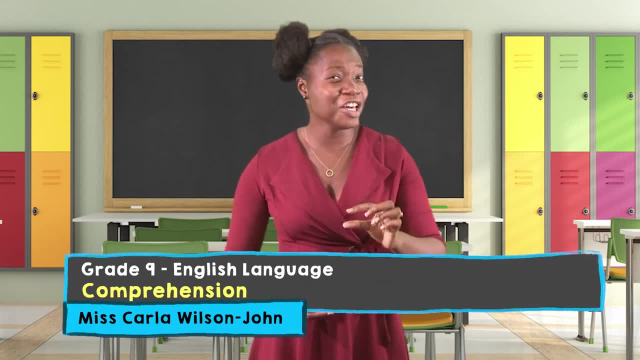 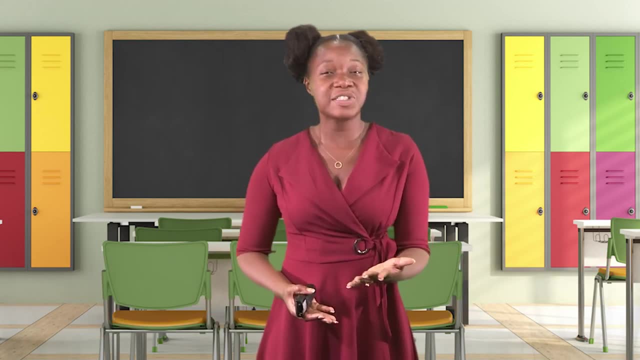 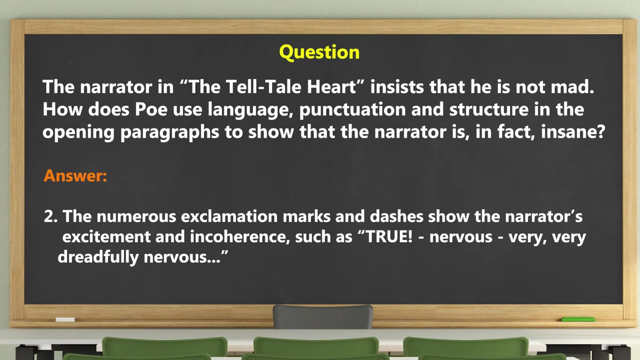 was his eye. Yes, it was this For one. the sentences are short, so we're thinking really fast. Note: some of the sentences do not even begin with capital letters. so there is no structure. There is no punctuation, There is no proper structure. There are several exclamation marks and dashes. We see that. 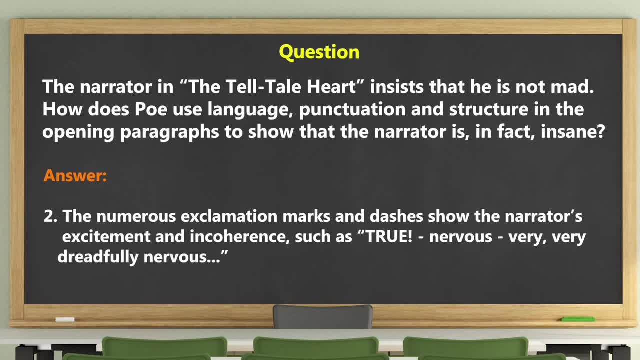 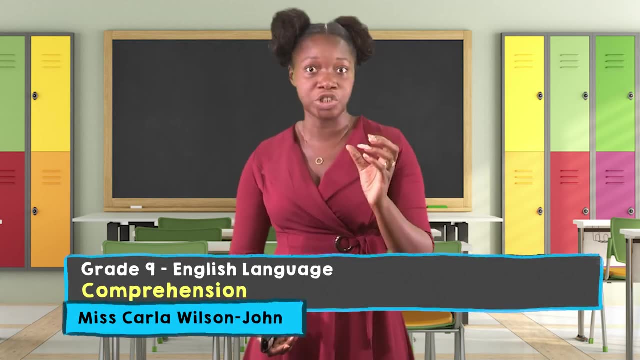 the narrator is excited. There is a bit of incoherence in how he speaks, True Nervous, Very, very dreadfully nervous. So you ought to imagine how he's expressing himself. Maybe his eyes begin to bulge out of his face. And finally, Poe's use of language.